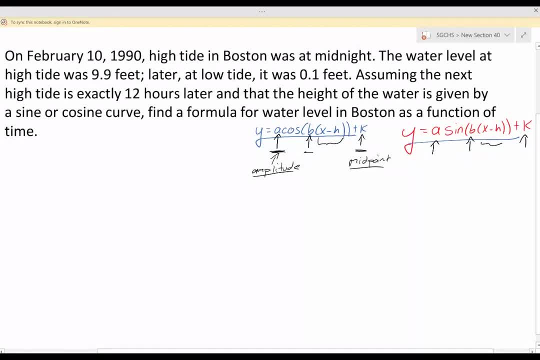 two things are both determined using the max or min points. Now our question here tells us that we have a high tide, of 9.9 ft- That is our maximum point- at 0.1 feet, or a low tide, which would be our minimum. So our max points? 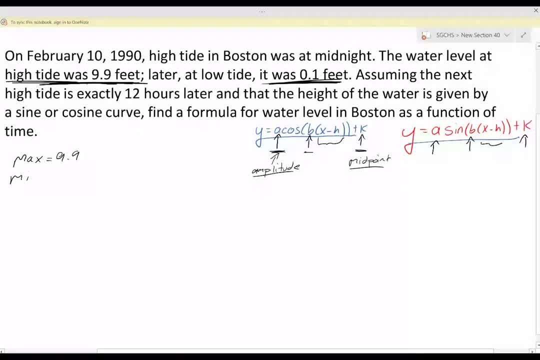 equals 9.9 feet and our min point equals 0.1 feet. Now understanding the equations that allow us to use these values to determine amplitude and min point are very useful. Amplitude, which is A, equals max minus min dividing by 2.. 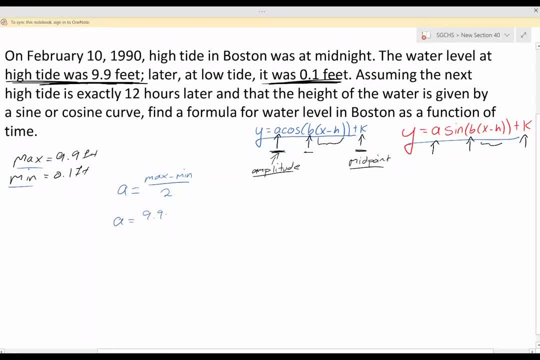 So that means 9.9 minus 0.1 divided by 2 will equal 9.8 divided by 2.. 9.8 divided by 2 gives us 4.9 feet. So we have an amplitude of 4.9 feet. So we will keep. 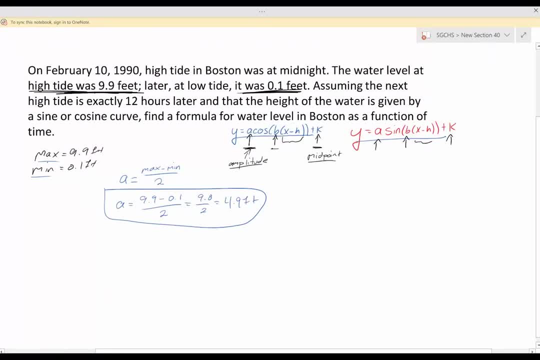 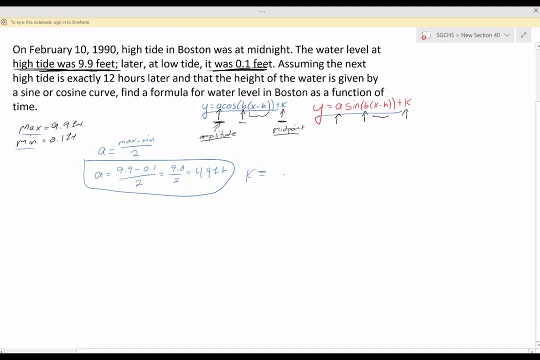 that in mind, We will keep that in our back pocket until we start graphing. Now, how about k? k is our midpoint Anytime you're finding midpoint, it's the sum of two numbers divided by 2.. So our midpoint here is between our max and our min, So that 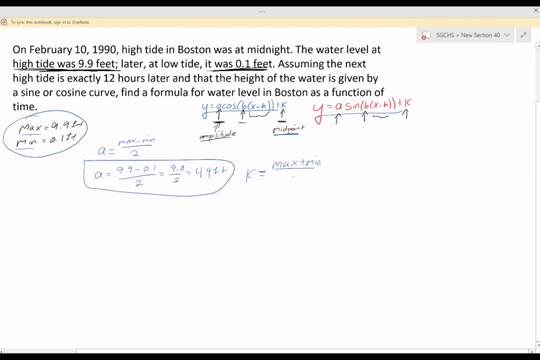 would be the sum of these two numbers, So max plus min divided by 2.. So 9.9 plus 0.1 divided by 2 gives us 10 divided by 2.. So that means k equals 5 feet. So now we have our midpoint and we have our amplitude, So we can start roughly. 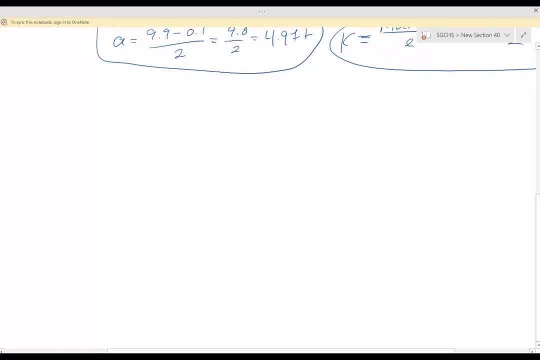 graphing this thing, So I'm not going to do any negative x-axis. That's because we're working in t hours, So it's our function of time. We can't have negative time, So this negative doesn't matter. Our minimum is 0.1 feet. 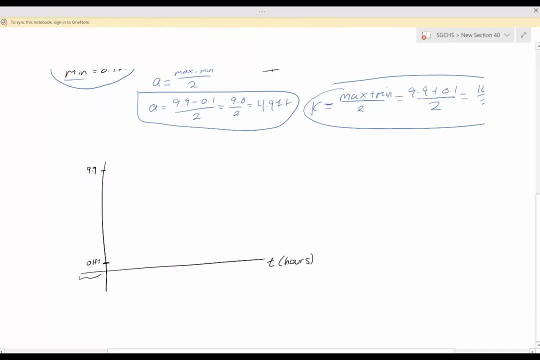 And our maximum is 9.9 feet. And again, that's from our high tide and our low tide. Let's maybe make that look a little nicer, I'm going to give titles to these axes. So this is height of tide And that is measured in feet, And this is time which is measured. 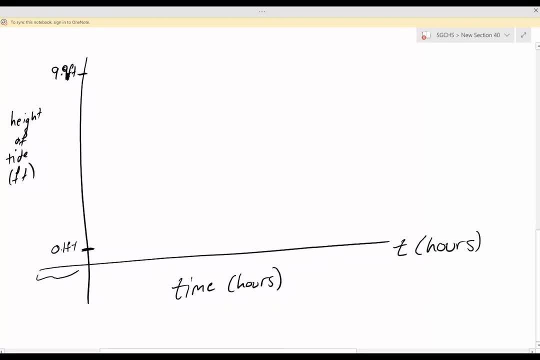 in hours. Now recognize we're not doing like a 12-hour clock, We're not doing 1 pm, 3 pm, We're doing kind of more army time. So this is 0 hours, which is also known as midnight. 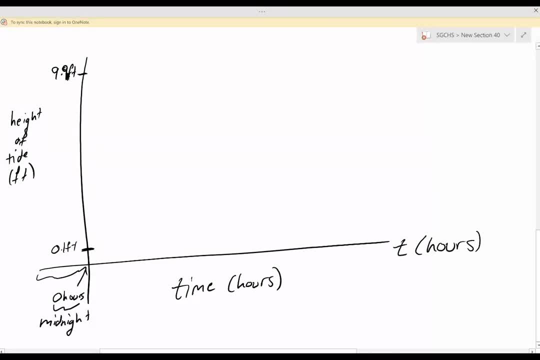 And then we'll just be increasing, So we'll be going to 6 hours, 12 hours, 14 hours, so on and so forth. We also have our midpoint, Which we know is 5 feet, So we can draw a rough line, just lining that out for us. And 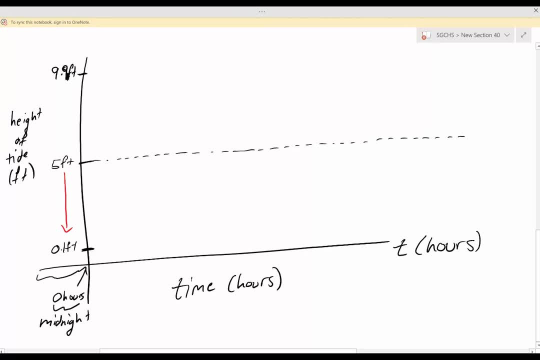 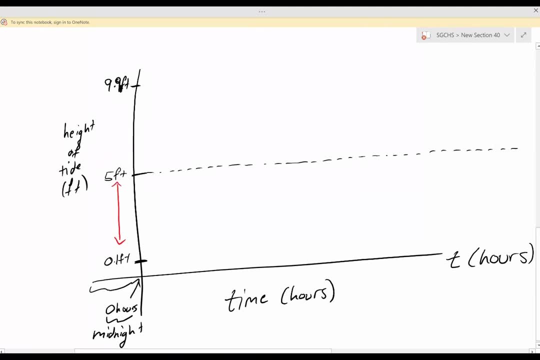 recognize that our amplitude here, which we figured out to be 4.9 feet, is true. To get from 0.1 to 5, that's 4.9 feet. The distance between 5 and 9.9 is also 4.9 feet, So that's. 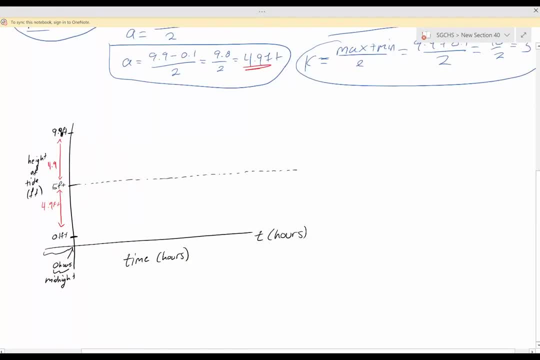 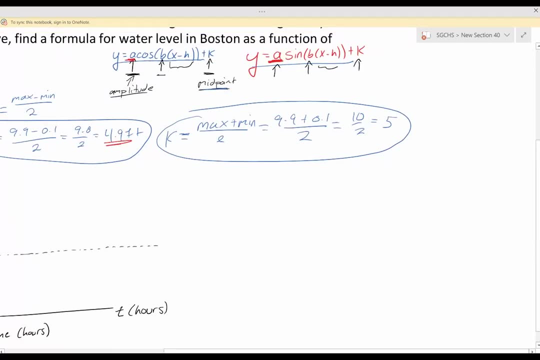 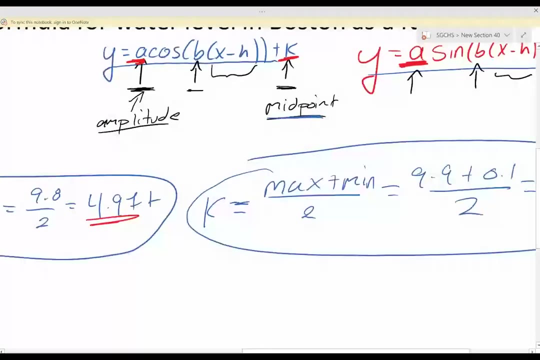 our amplitude, So we already have a few values that we can plug into our equations of performing this. We have A and we have K, And remember, these are the same regardless if you're dealing with cos or sin. Now, the other one that they have in common is b, which is tied to the period of what? 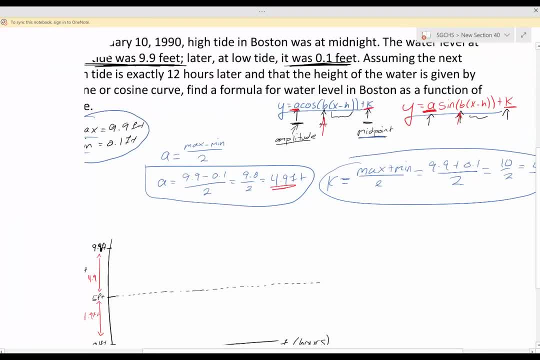 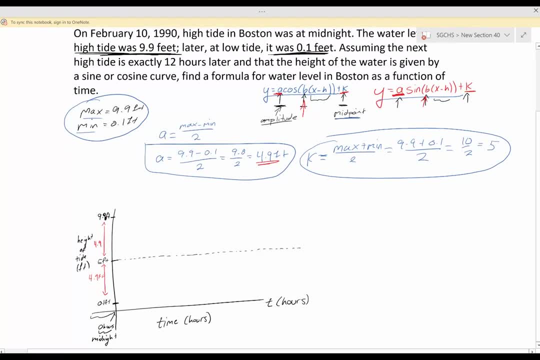 is occurring Now. whenever you're dealing with real-world problems or work with real-world problems, you have to stick to your problem: Okay Announcement or word problems. when you're trying to graph or form an equation, your y-intercept is usually: 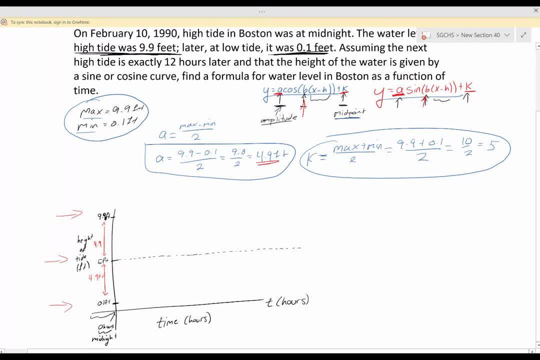 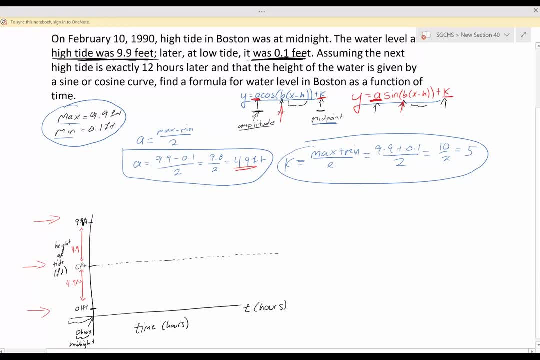 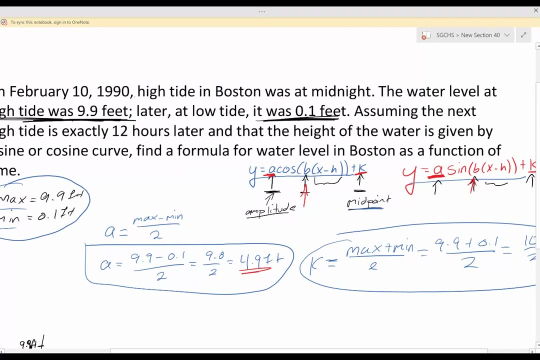 either a maximum, a midpoint or a minimum, Not always, but 90% of the time. it's useful to graph it saying that's where our y-intercept is. Now, if we read our question again, it says high tide in Boston was at midnight. 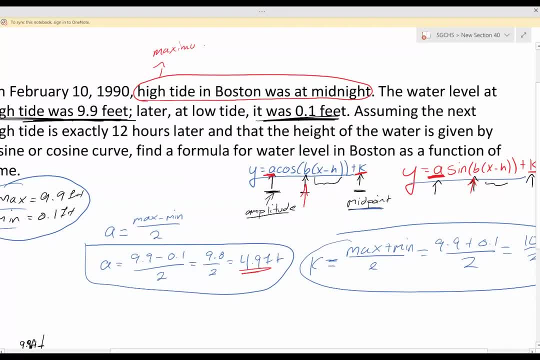 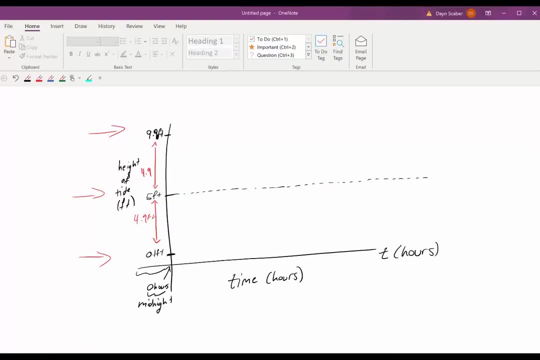 That means we're at a maximum at midnight, which is zero hours. Remember, our maximum is 9.9 feet, So that means when we're at zero hours, we're at 9.9.. So our y-intercept is a maximum point found here. 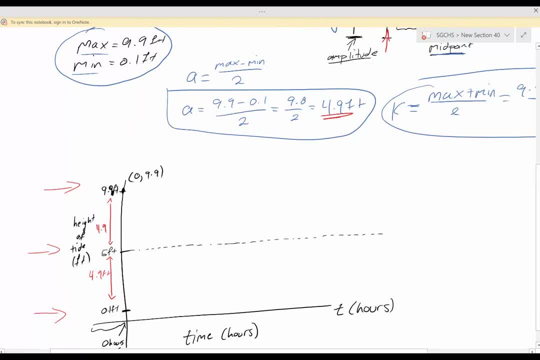 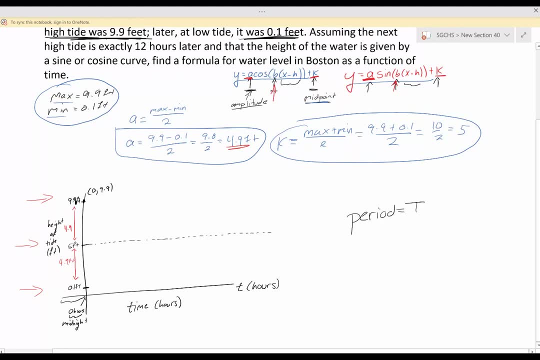 So this is zero and 9.9.. Now, if we want to start determining what b is, we have to determine what the period is, And remember, the period equals t. The reason we have to figure out the period is because we can figure out what b is. 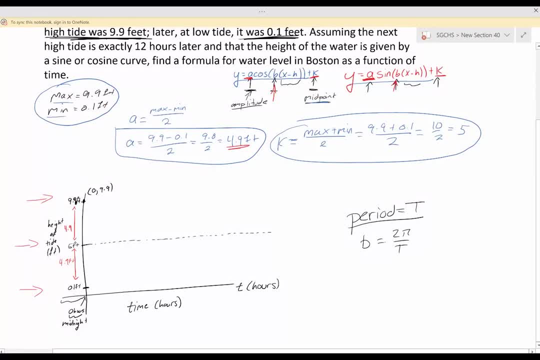 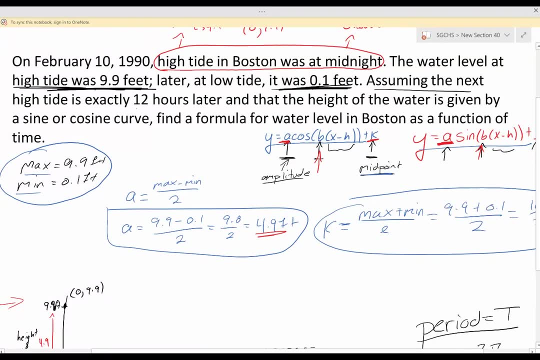 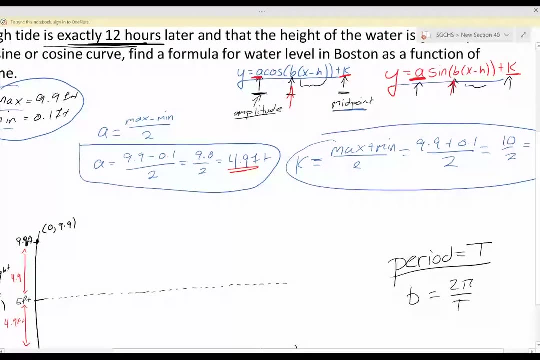 by the relationship of two pi over t. Now, if we go back to our question, it tells us, assuming the next high tide is exactly 12 hours, Remember maximums and minimums. repeat for the period time. So if our next high tide is 12 hours, that means our next. 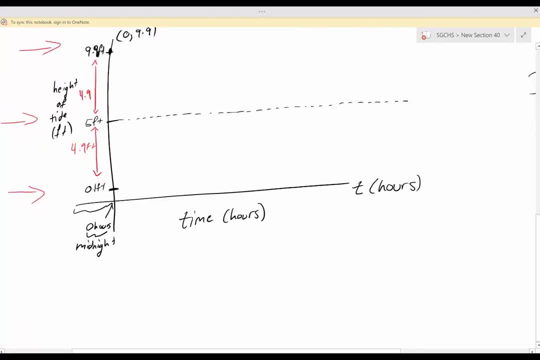 maximum is at 12 hours, So we could maybe write this as 12 here, 12 hours, and we have a maximum point there. So there is 12 and 9.9.. Another 12 hours after that, which would be 24 hours. 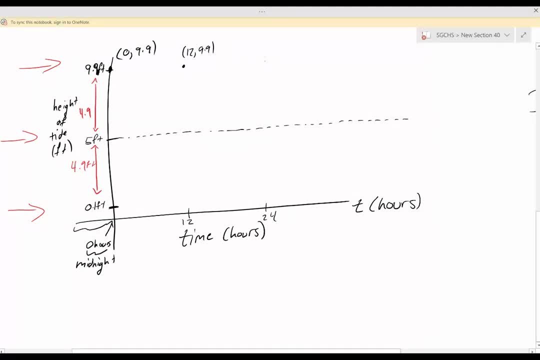 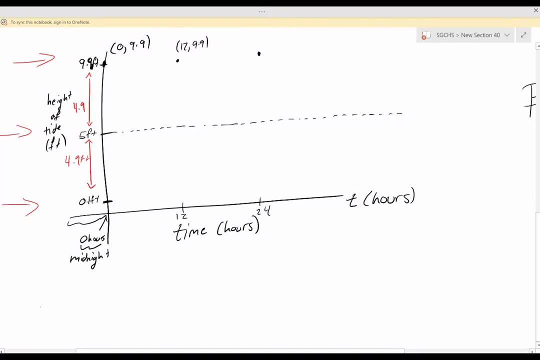 you're going to get another maximum. So now we have a few points plotted. Something really useful to understand is min points, mid points, minimum points are directly in the middle of two adjacent max points. So mid points or minimum points. 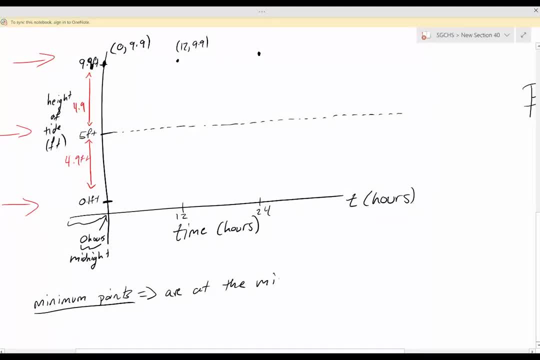 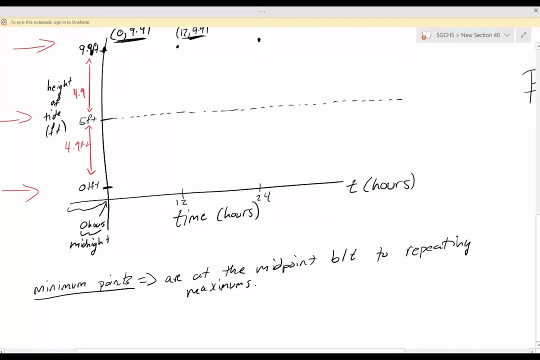 are at the midpoint between two repeating maximums. So that means our midpoint between our 0 and 9.9 maximum and 12 and 9.9 maximum will be directly in the middle of 0 and 12.. So to find a midpoint it's always the two numbers. 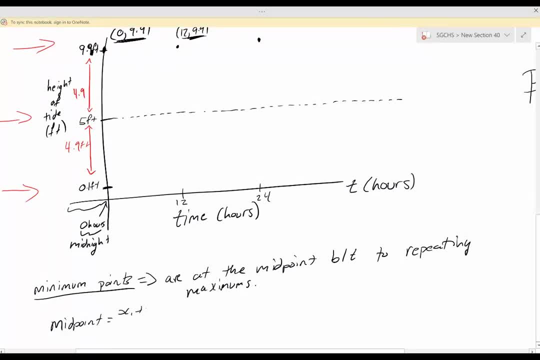 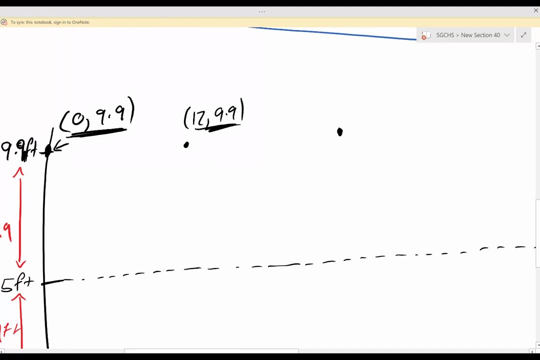 that you're determining. So let's say x1 plus x2 and divide it by two. You can kind of think about that in terms of how that relates to finding your midpoint for k. So we want to find the midpoint between this maximum and this maximum. 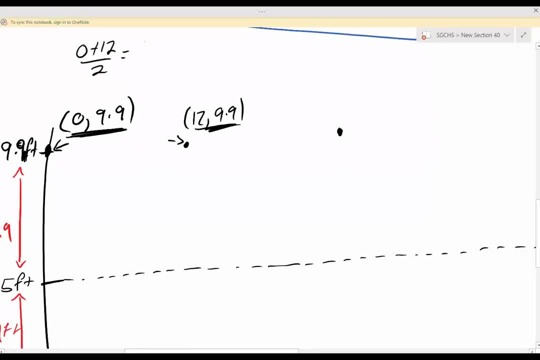 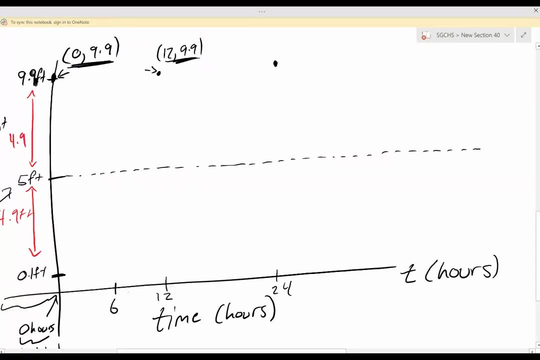 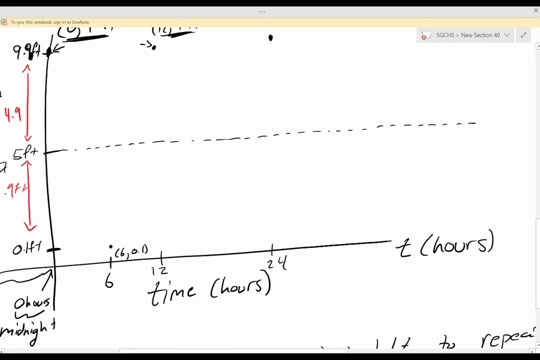 So 0 plus 12 divided by two gives us 12 divided by two, which is six. So that means our midpoint will be found at six here. So we have a point here now which is six and 0.1.. Now recognize. 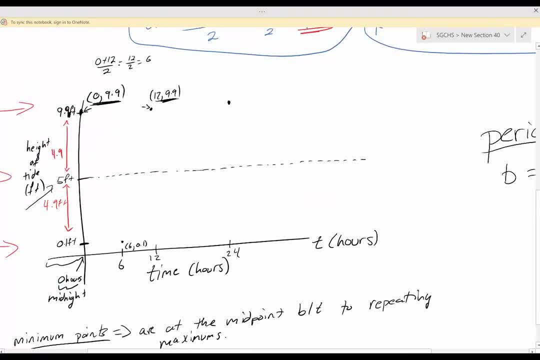 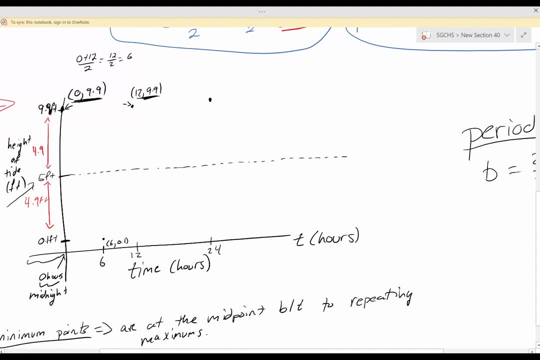 midpoints or minimum values occur for the period. Okay, so we know our period is every 12 hours, So our next minimum will occur 12 hours after six, which is 18.. So here we have 18 and 0.1.. 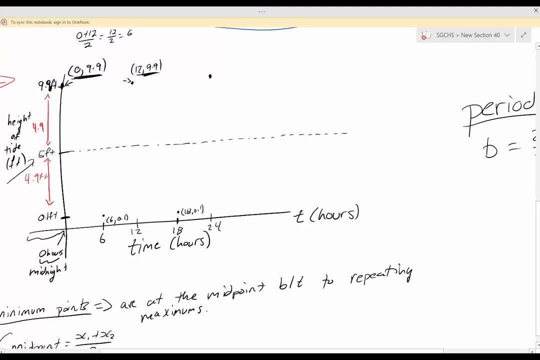 Something kind of useful to kind of notice is we could also find this using our midpoint equation. So 12 plus 24 divided by two, 12 plus 24, gives me 36, and dividing that by two gives me 18.. So you could also determine it that way. 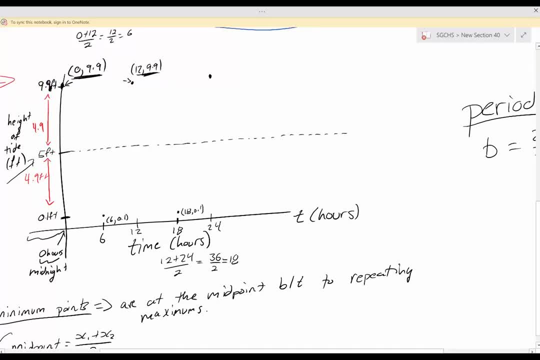 Now, at this point, whenever you have your maximum and your minimum values, you can now roughly form the equation. Okay, so we're going to go down, go up and repeat this process. So now you can see that we're going to be able to find our midpoint. 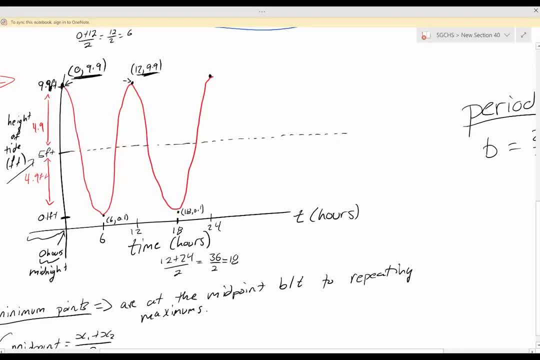 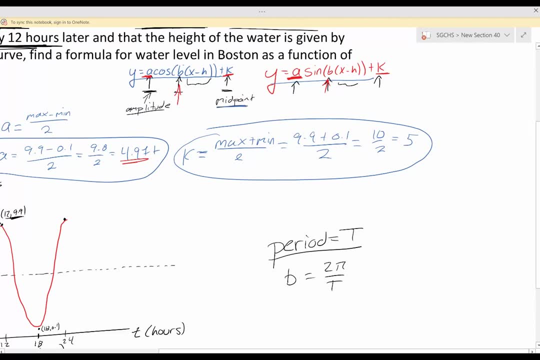 So now you can see that we're going to be able to find our midpoint. So now you can see that we're going to be able to find our midpoint, that we're starting to form a nice cos or a sine function. Now we have A, we have K. 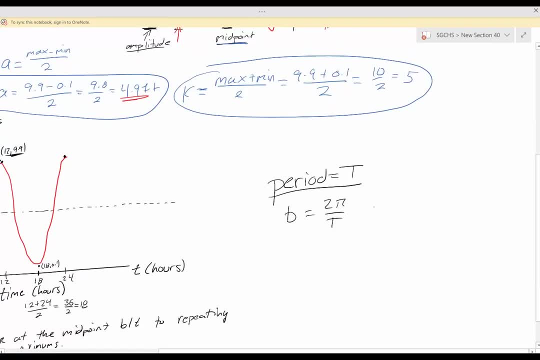 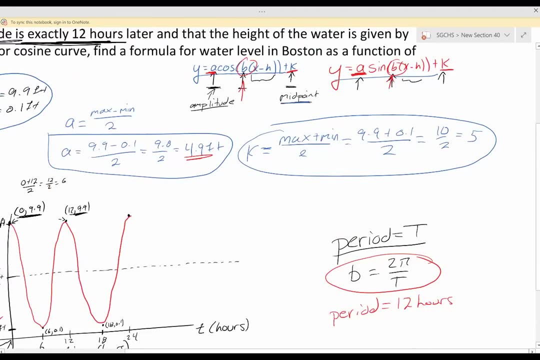 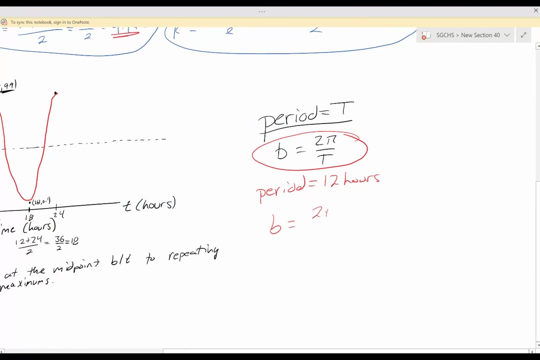 How do we determine what B is? Well, B is simply related to the period. Remember, the period in this case is every 12 hours. Okay, Your maximums, your high tides repeat exactly 12 hours apart. So here B will equal two pi divided by 12.. 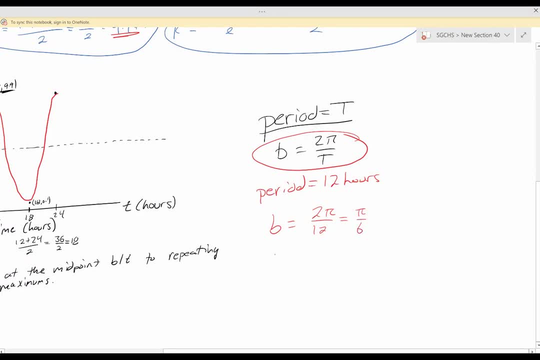 So here: B will equal two pi divided by 12.. And you can now simply So: here: B will equal two pi divided by 12, and you can now simply simplify that to pi over 6.. So b equals pi over 6.. So let's write out our equations that we have. 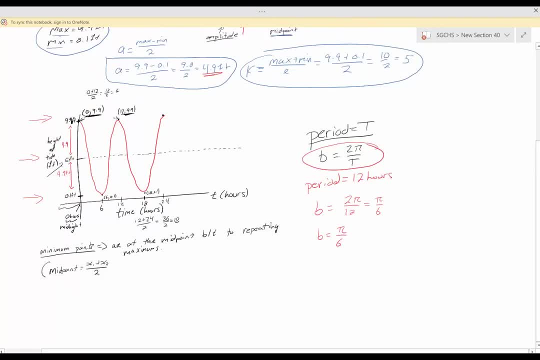 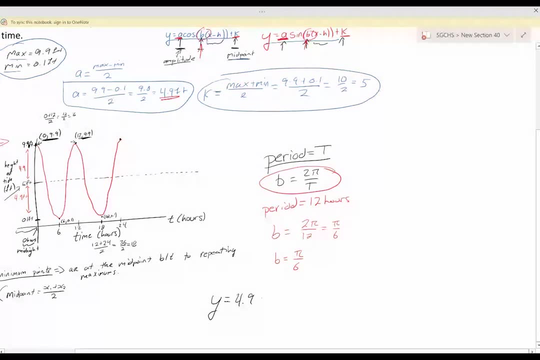 so far. If we were to write it in a cos function, it would be y equals a, which we figured out was 4.9 cos b, which is pi over 6, x minus h plus 5, which is k, If we did it for our sine function. 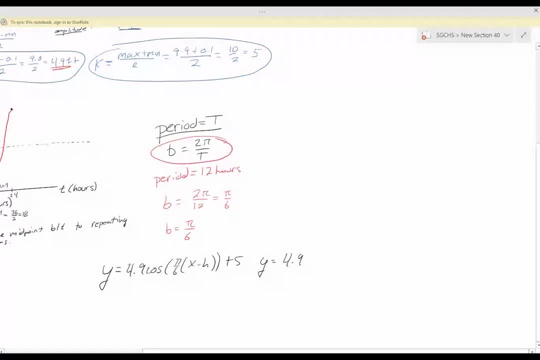 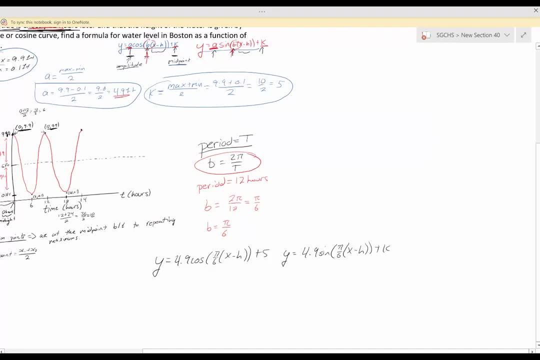 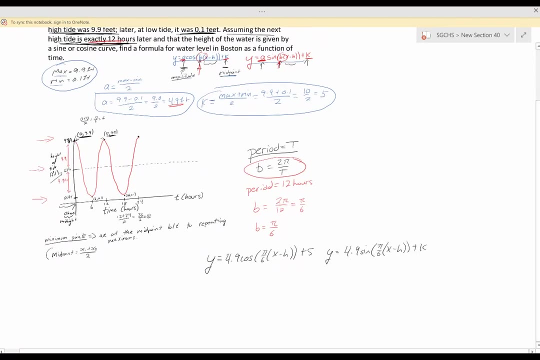 it's going to be the same thing, simply with sine 4.9, sine pi over 6, x minus h plus k. Now, at this point we can start solving for those phase shifts. Now remember phase shifts, so that h value is unique, depending. 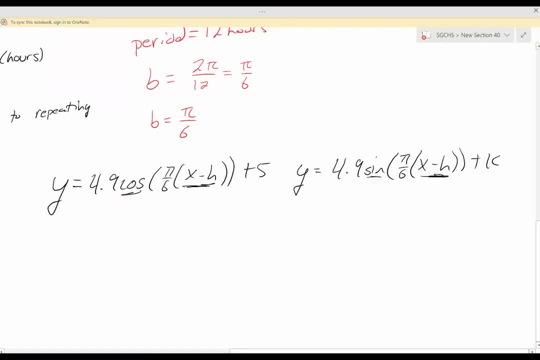 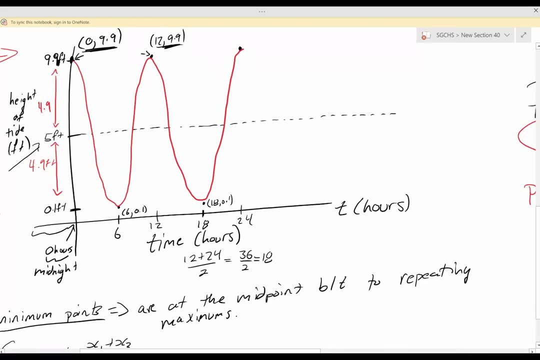 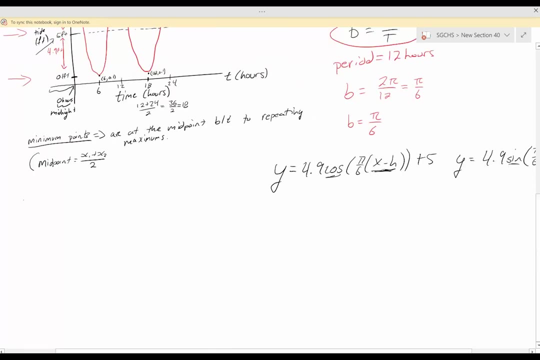 on your sine and cos. There's infinite amount of h values that we can put in here, but we'll talk about that right now. So in order to figure out what the phase shift is, we need to know what our base functions look like. So our base functions. what I mean by that is what does y equals cos x. 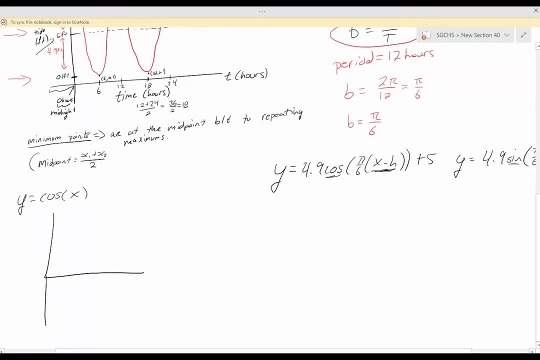 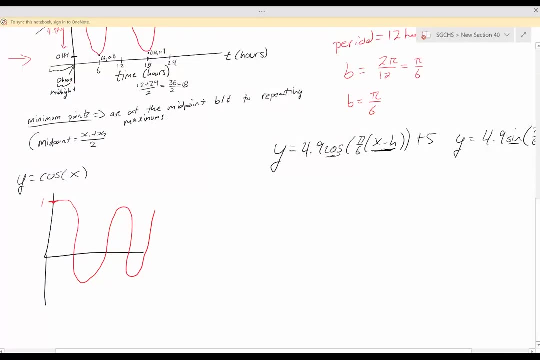 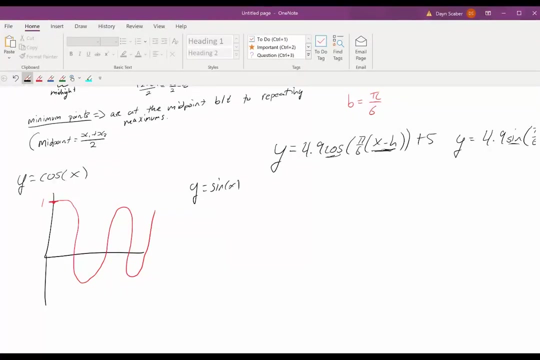 look like. Okay, and at this point you should understand what these look like. Cos x starts at a maximum of 1.. Okay, so we just need the rough idea of what cos x is. Sine x- starting point. what I mean by that is, your y-intercept starts at the midline, So 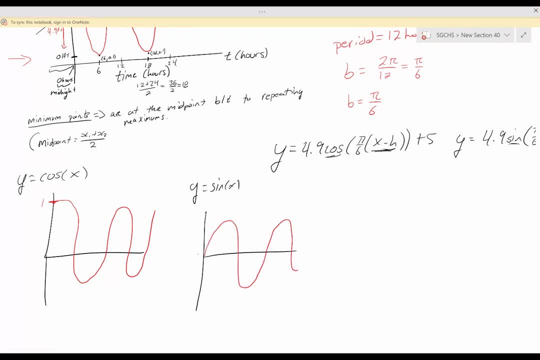 right here. Now what we're going to do is we're going to look at our new equation and figure out: okay, where did our starting point shift to for cos x And where did our starting point shift to for sine x? Let's first focus on cos x. So remember cos x starting point. 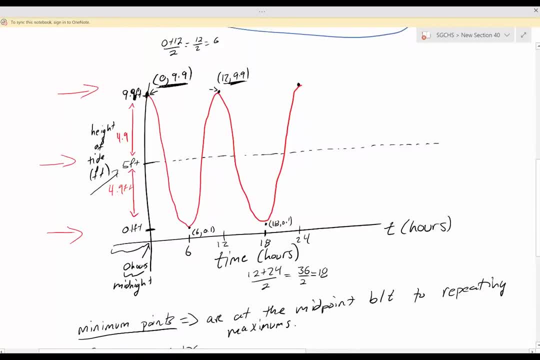 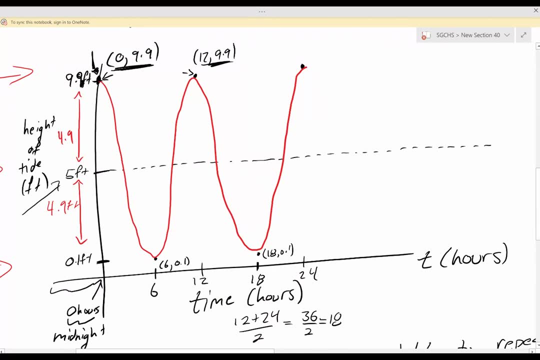 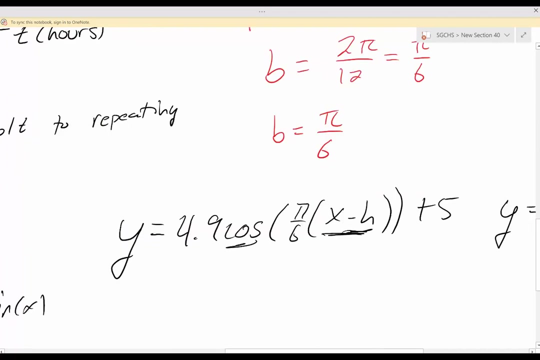 is a maximum. Where did that maximum go? So, if we look up here, our maximum never actually moved. Our maximum here has stayed and our y-intercept is still a maximum. We could also use this maximum as a phase shift. We could see as if cos shifted 12 units to the right. So we could either represent cos. 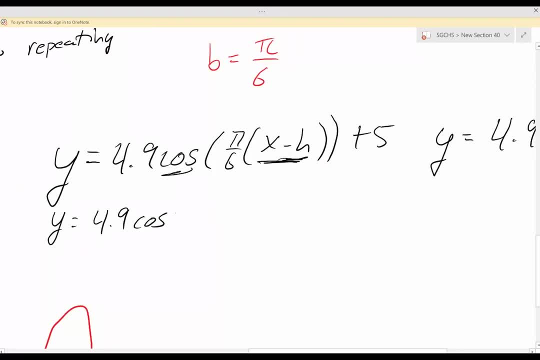 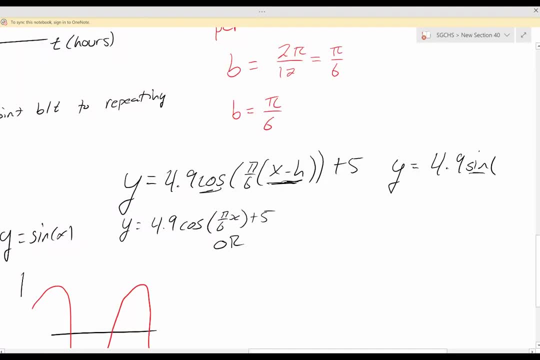 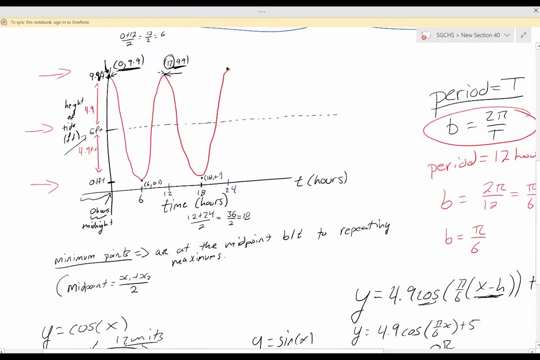 as if we had no shift at all. so simply pi over 6 times x plus 5, or we could see as if our starting point here 12 units over to the right. So because of this here. So that means we could also represent this. 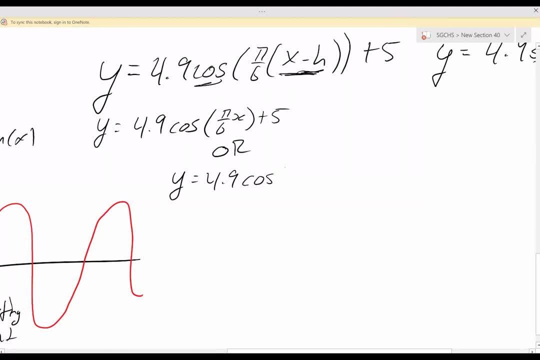 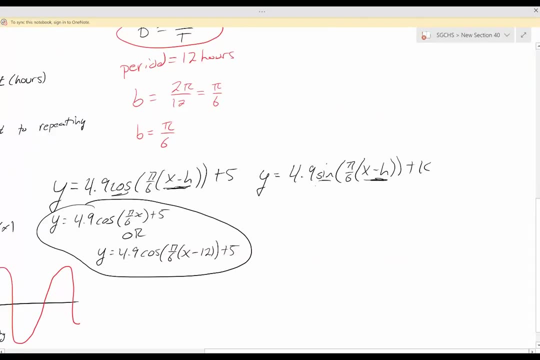 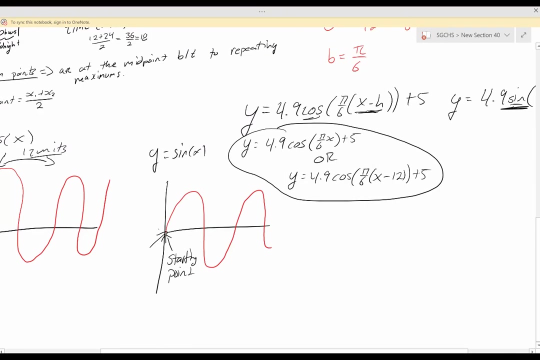 as y equals 4.9 cos pi over 6, x minus 12.. There's two solutions there which will graph the same equation in terms of cosine. Now, what about the sine function? Well, sine function, our starting points- is at the midline, So we have to find. 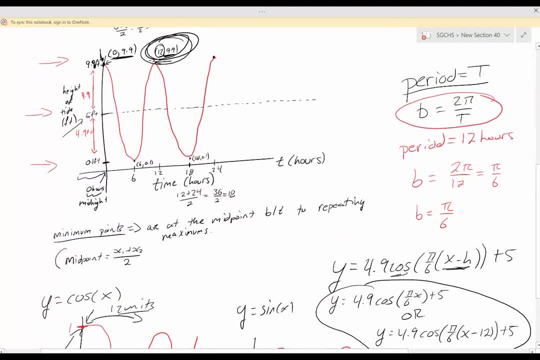 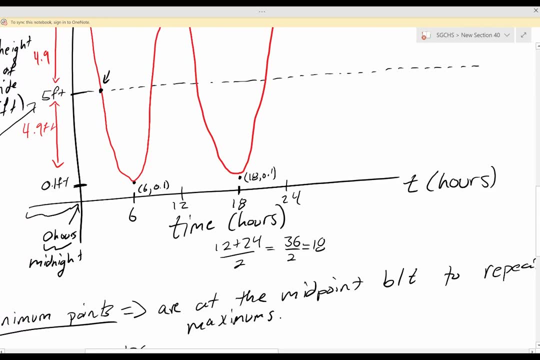 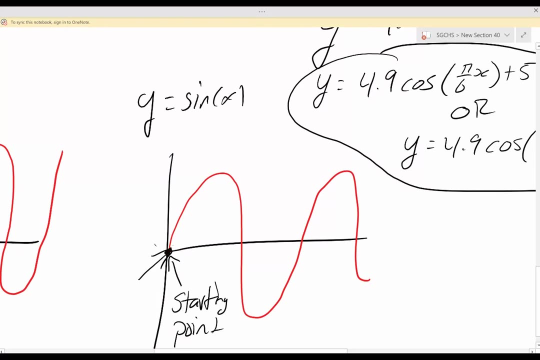 midline points on our equation and figure out how far it is from the x or the y axis. So here we have a midpoint, but that midpoint doesn't quite work because recognize on our base sine function, our starting point: as it goes to the right, it increases. 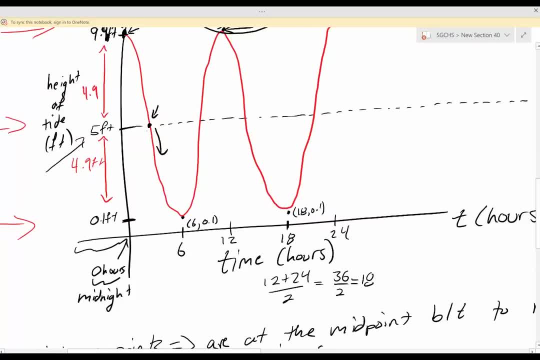 Here it decreases. You could still technically use this midpoint, but you would have to apply a reflection, which I won't be doing here. So this midpoint doesn't quite work without reflection. So what I'm going to use is this midpoint, If you can kind of compare it to our sine function here. 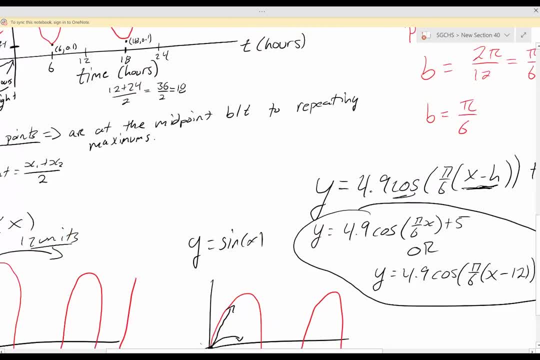 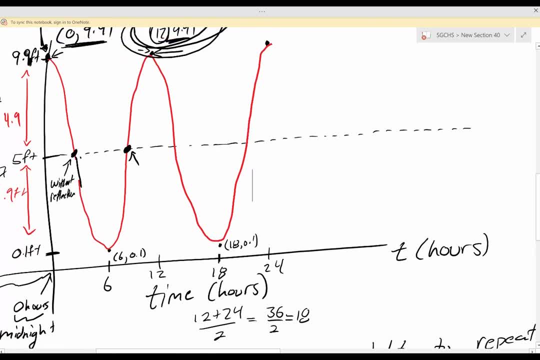 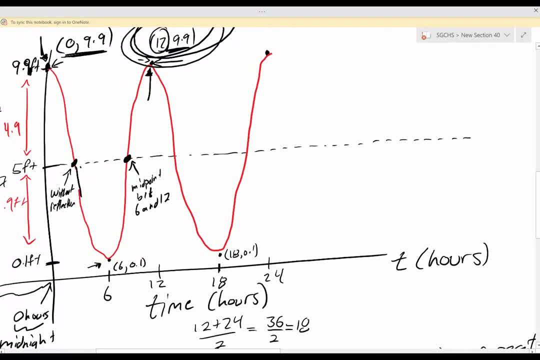 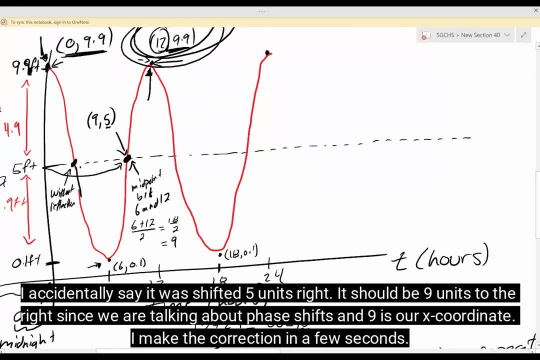 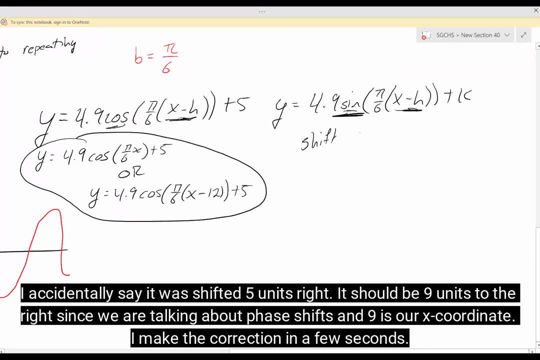 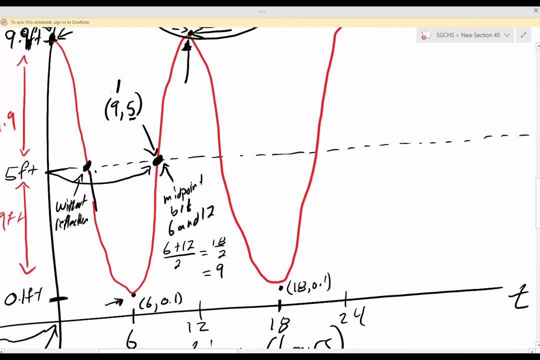 shift over five units to the right. So now we can write that in our equation. So if we shift five units to the right, then we'll have x minus five or- sorry, not five, my bad- It'll be nine units to the right. 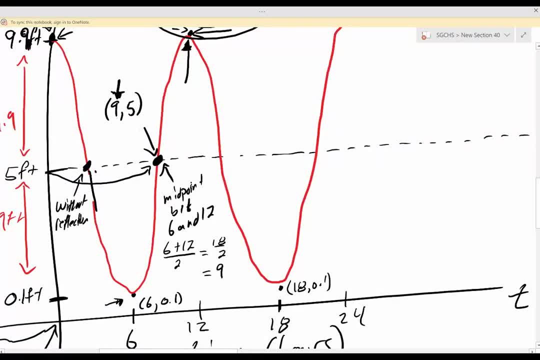 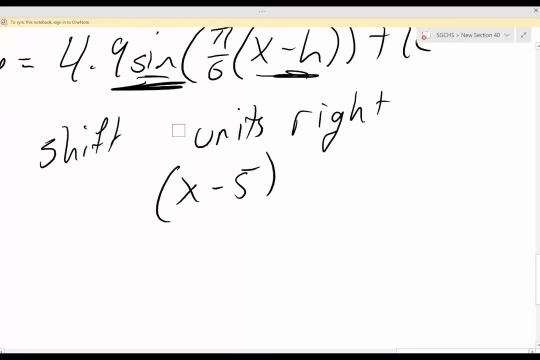 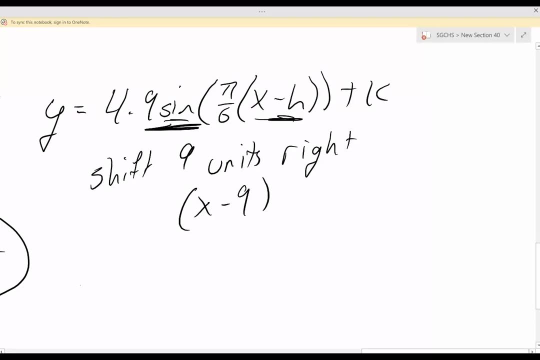 I was looking at the y-coordinate, but we're talking about the x-coordinate. So nine units to the right. So we have shifted nine units to the right, So now we can plug those in to our equation. So y equals 4.9 sine pi over six x minus nine. 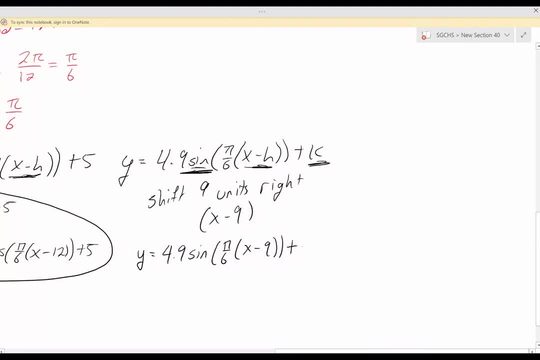 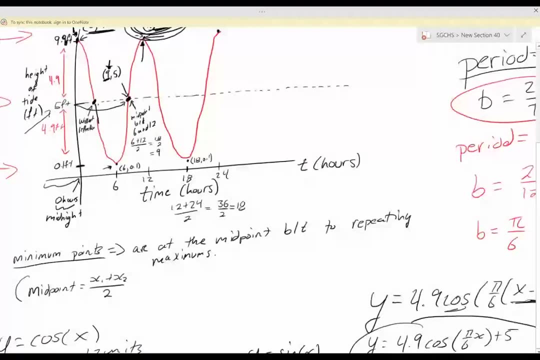 plus forgot to put my k value here, which is okay, which is simply five, because that's our minimum value, That's our midline, So I hope that was helpful. Again, let's maybe look at how would we represent it using this midpoint.